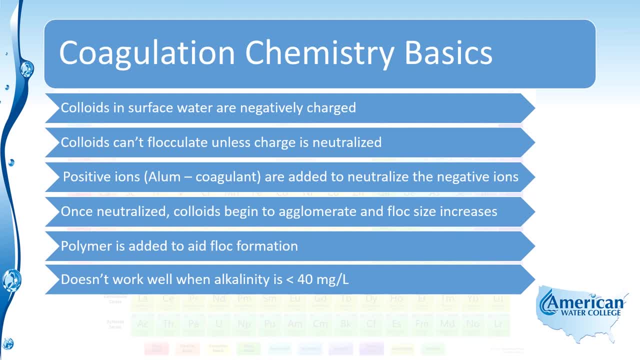 hydroxide which looks kind of like a snowflake in the water, And that aluminum hydroxide flock will then act to neutralize the colloids or attract the colloids to it and form even larger flock. So aluminum sulfate and ferric sulfate require alkalinity in the water in order for them. 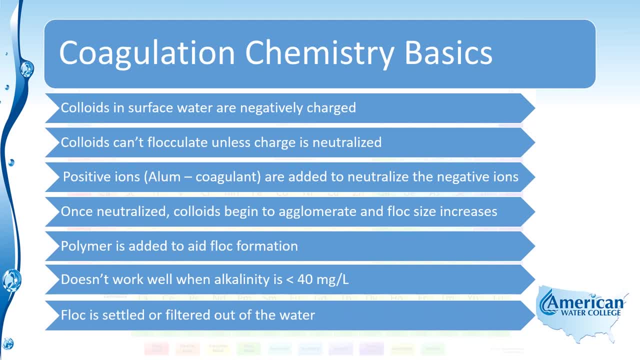 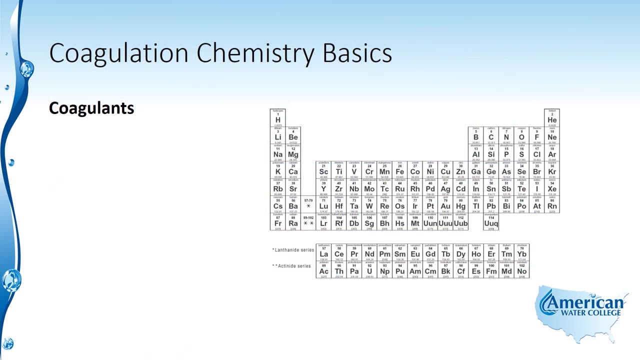 to be effective. Well, once the flock has formed to a size large enough to settle out, it is settled in the sedimentation basin or filtered out in the filtration process. Most treatment plants use trivalent coagulants Because trivalent coagulants are 50 to 60 times more effective than bivalent coagulants. 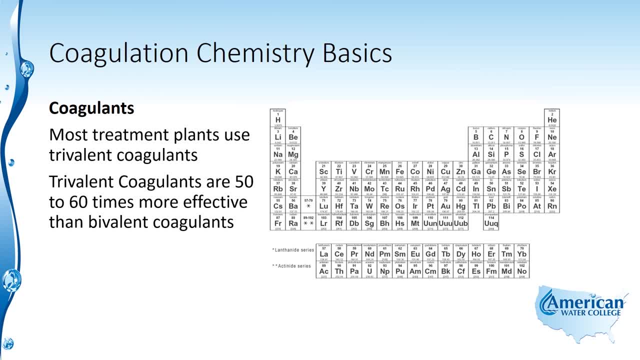 Now, what we mean by trivalent coagulants is that those are coagulants that have three positive charges associated with them. A bivalent coagulant only has two positive charges and a monovalent coagulant only has one positive charge, And trivalent coagulants are a thousand. 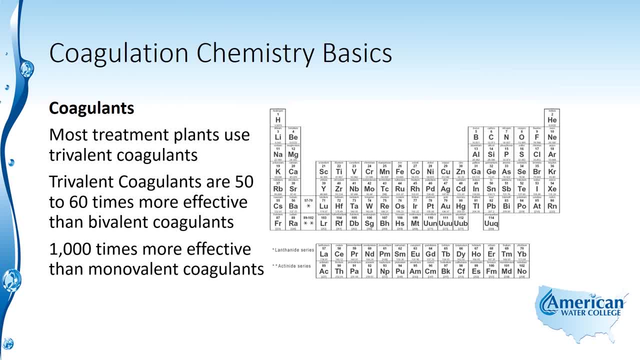 times more effective than monovalent coagulant. Aluminum is a trivalent coagulant and so is iron, So you have your aluminum salts or your aluminum sulfate as a coagulant. You also have several iron salt coagulants: ferric chloride, ferrous sulfate and ferric sulfate. So aluminum and iron are trivalent. 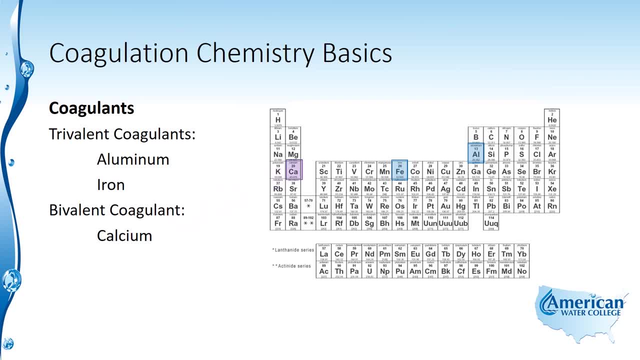 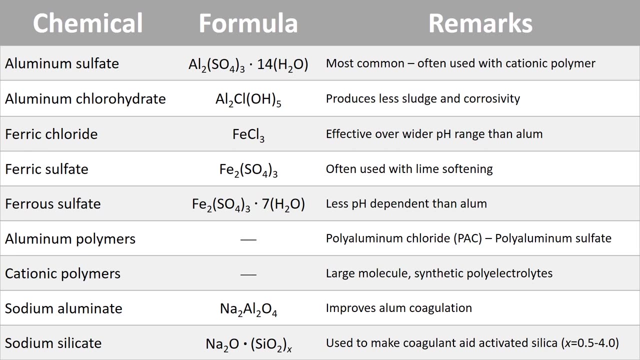 coagulant. An example of a bivalent coagulant would be calcium hydroxide and a monovalent coagulant would be sodium silicate. Now let's look at this chart that shows us the different coagulants that are commonly used. First is aluminum sulfate. Aluminum sulfate is the most. 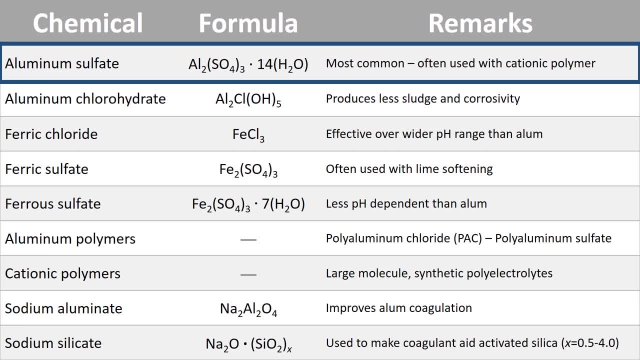 commonly used coagulant and it's often used in conjunction with a cationic polymer. A cationic polymer is a polymer that gives off positive ions once it's dissolved in water. Next is aluminum chlorohydrate. It's again aluminum based and it produces less sludge. 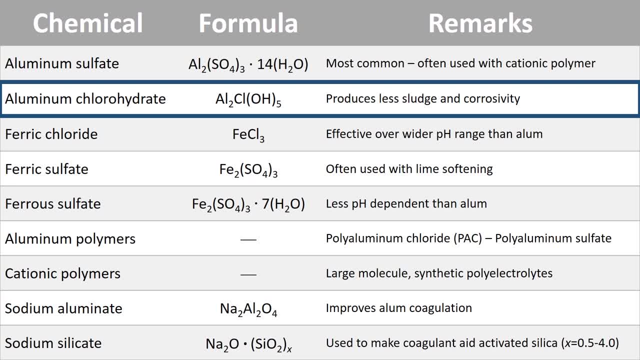 and is less corrosive than aluminum sulfate. Ferric chloride is the first of our iron salt coagulants and it's effective over a wider pH range than alum, So there are some applications where ferric chloride might be used rather than alum. However, 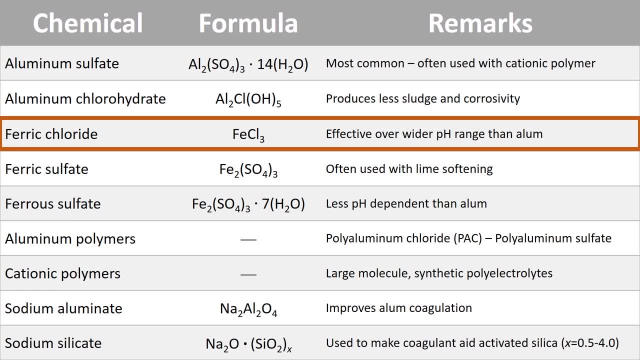 it is very corrosive and it tends to stain the water treatment plant, a rust color Ferric sulfate is similar to aluminum sulfate in that it requires alkalinity in order for it to be effective, or at least alkalinity above 40 milligrams per liter. So it's a very corrosive. 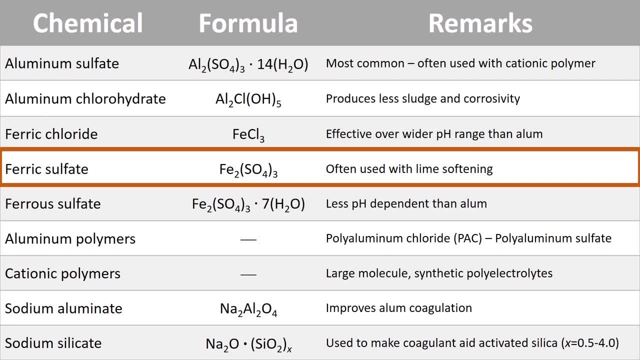 process that require a lot of Rogan ethical solvents as well as a number ofいるic sulfates. So that is how far prosecuted alum is packaged, And ferric sulfate is often used as part of the lime softening process. so something you 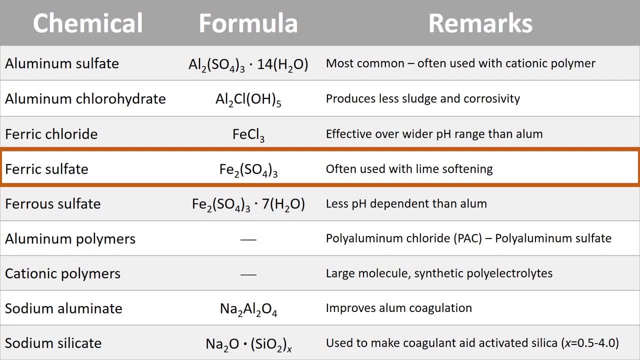 want to remember for your test is that ferric sulfate is often used with lime softening. Ferrous sulfate is less pH dependent than alum similar to ferric chloride. Then there are some aluminum polymers. one particular aluminum polymer is called polychloride. This is closer to Columb stores, One particular aluminum polymer. 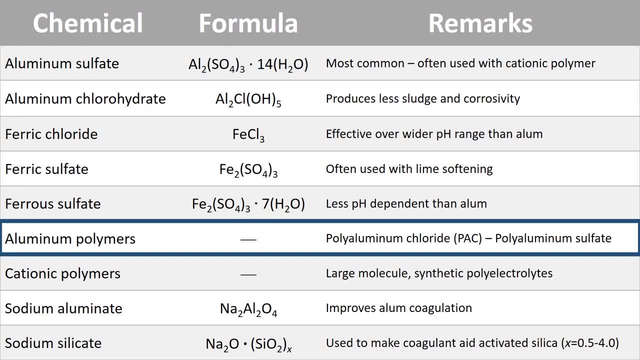 is called polychloride, and this is classed as Borax. Butcówanol is called polyaluminum chloride or PAC, and another is polyaluminum sulfate. Next on our list are cationic polymers, and these are large molecule synthetic polyelectrolytes. 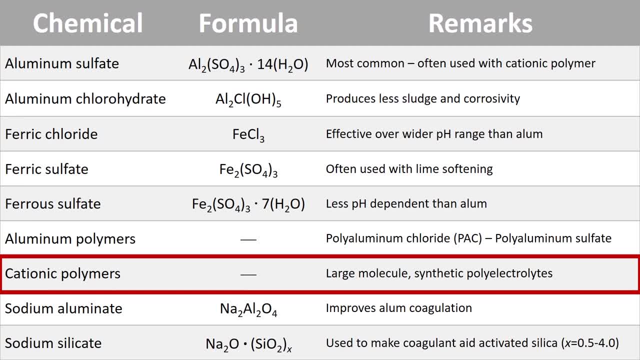 So these are man-made products- is where aluminum sulfate and the ferric salts are naturally occurring. Next is sodium aluminate, which is often used along with alum because it improves the alum coagulation process. And then, finally, we have sodium silicate, which is used to make the coagulant aid activated silica, So sodium. 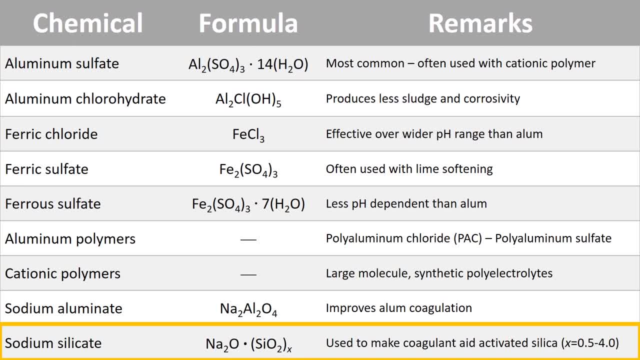 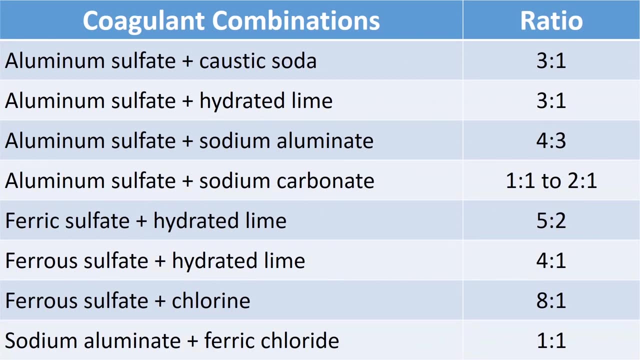 silicate is used by water treatment plant operators to make activated silica, which is added in addition to a primary coagulant to enhance the coagulation process. Well, this chart shows the different combinations of chemicals that can be used with coagulants.